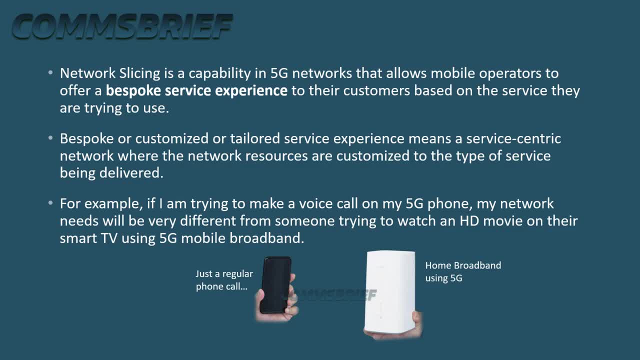 Network slicing is a capability in 5G networks That allows mobile operators to offer a bespoke service experience to their customers based on the service they're trying to use. Bespoke or customized or tailored service experience means a service-centric network where the network resources are customized to the type of service being delivered. 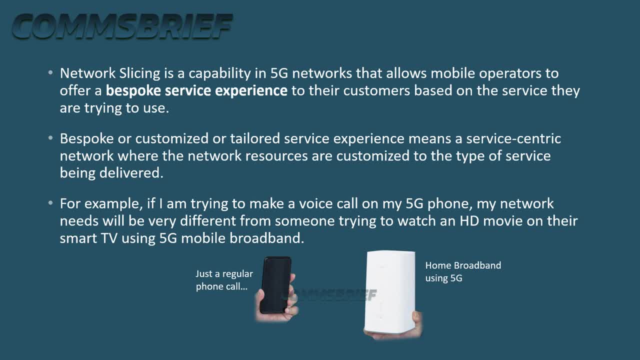 For example, if I'm trying to make a voice call on my 5G phone, my network needs will be very different from someone trying to watch an HD movie or a 5G video. So if I'm trying to make a voice call on my 5G phone, 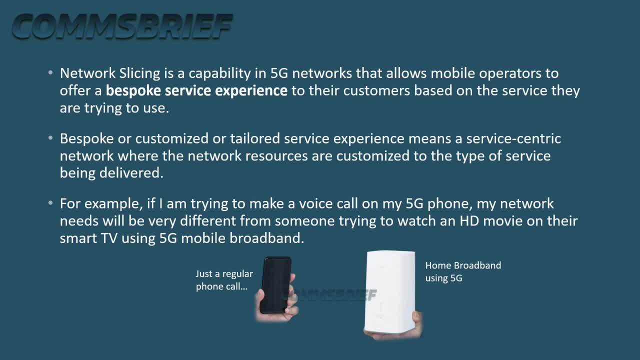 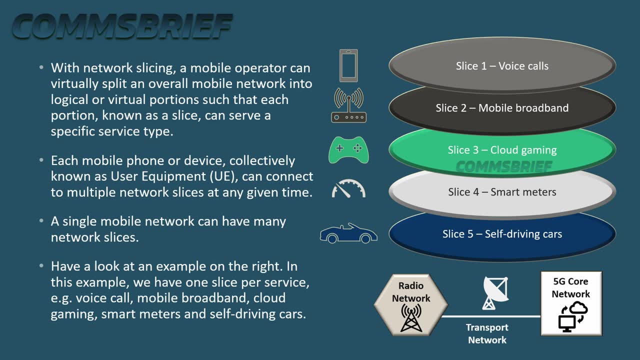 I'm going to be doing a voice call on their smart TV using 5G mobile broadband. With network slicing, a mobile operator can virtually split an overall mobile network into logical or virtual portions, such that each portion known as a slice can serve a specific service type. Each mobile phone or device collectively known as 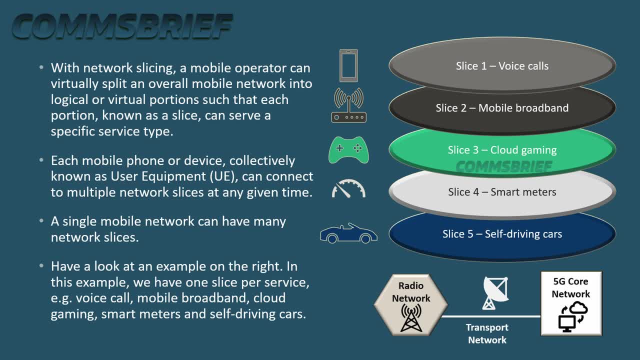 user equipment. UE can connect to multiple network slices at any given time. at any given time, a single mobile network can have many network slices. have a look at an example on the right. in this example we have one slice per service, for example, voice call, mobile broadband. 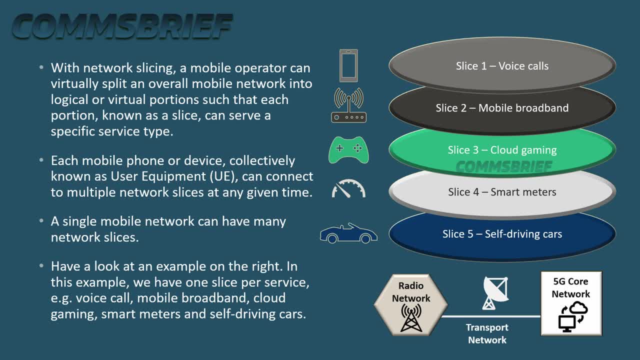 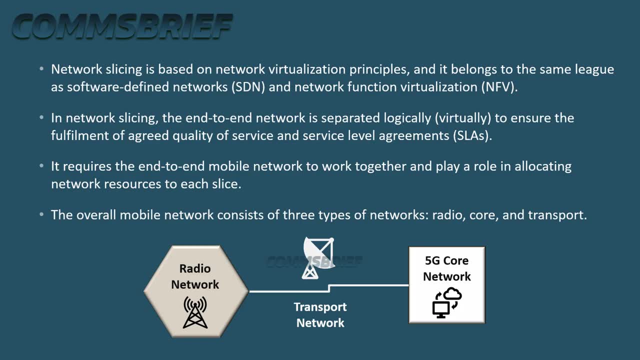 cloud gaming, smart meters and self-driving cars. network slicing is based on network virtualization principles and it belongs to the same league as sdn software defined networks and nfv network function virtualization. in network slicing, the end-to-end network is separated logically virtually to ensure the fulfillment of agreed quality of service, qos and service level agreements- slas. 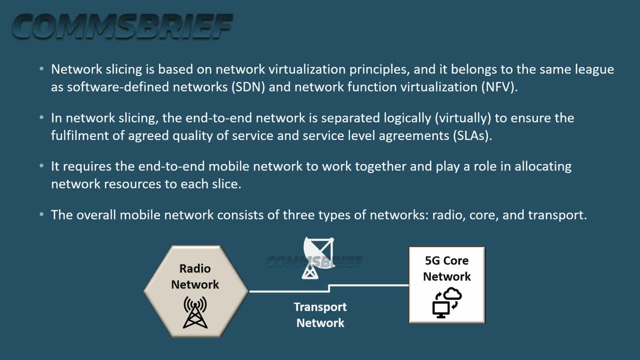 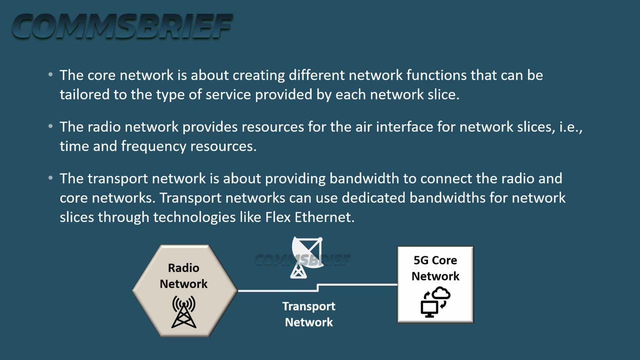 it requires the end-to-end mobile network to work together and play a role in allocating network resources to each slice. the overall mobile network consists of three types of networks: radio network, core network and transport network. the core network is about creating different network functions that can be tailored to the type of service provided by each network. 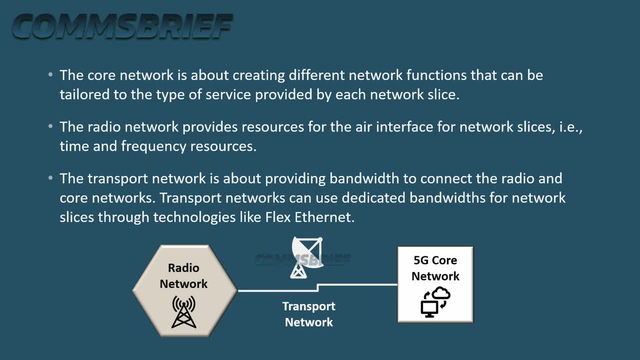 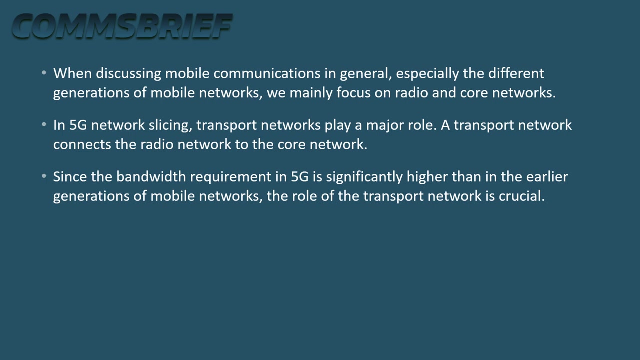 slice. the radio network provides resources for the air interface for network slices, that is, time and frequency resources. the transport network is about providing bandwidth to connect the radio and core networks. transport networks can use dedicated bandwidths for network slices through technologies like flex ethernet. when discussing mobile communications in general, especially the different generations of 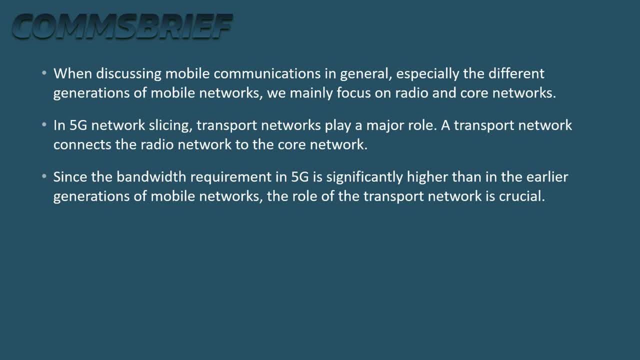 mobile networks, we mainly focus on radio and core networks- core networks. In 5G network slicing transport networks play a major role. A transport network connects the radio network to the core network. Since the bandwidth requirement in 5G is significantly higher than in the earlier. 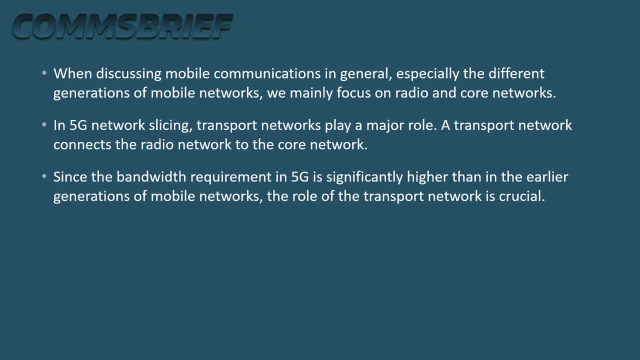 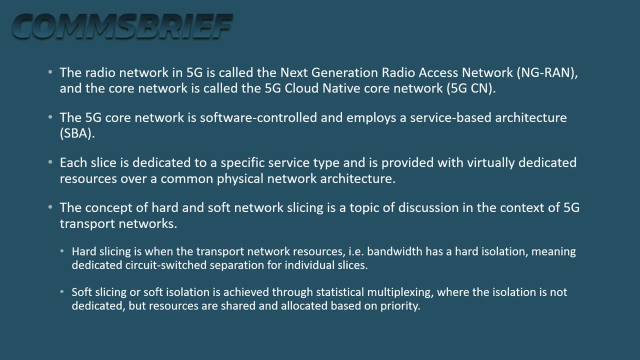 generations of mobile networks, the role of the transport networks is crucial. The radio network in 5G is called the Next Generation Radio Access Network and the core network is called the 5G Cloud Native Core Network. The 5G core network is software controlled and employs a service-based architecture. 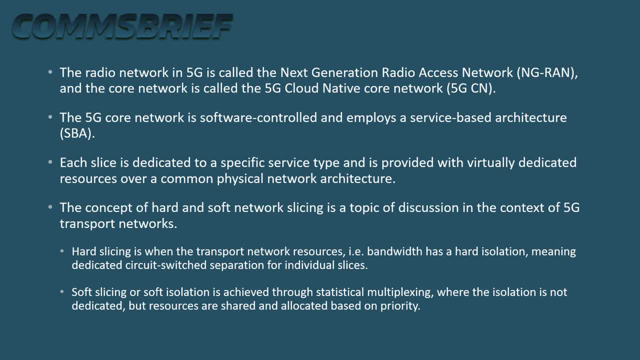 Each slice is dedicated to a specific service type and is provided with virtually dedicated resources over a common physical network architecture. The concept of hard and soft network slicing is a topic of discussion in the context of 5G transport networks. Hard slicing is when the transport network resource has a hard isolation. 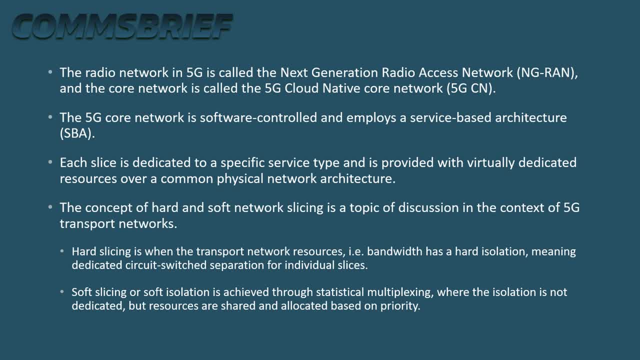 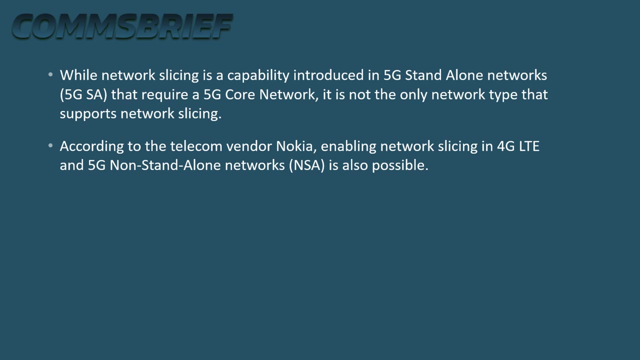 meaning dedicated, circuit-switched separation for individual slices. Soft slicing, or soft isolation, is achieved through statistical multiplexing, where the isolation is not dedicated but resources are shared and allocated based on priority, While network slicing is a capability introduced in 5G standalone networks that require 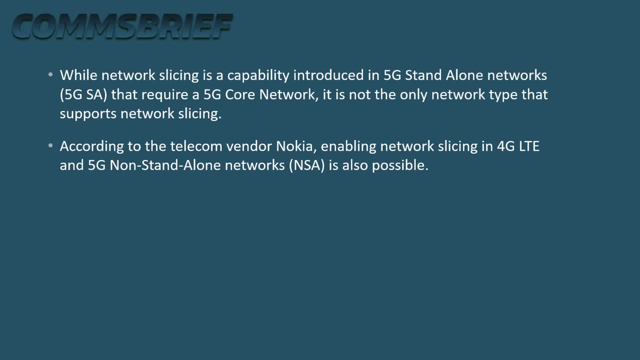 a 5G core network. it is not the only network type that supports network slicing. According to the telecom vendor Nokia, enabling network slicing in 4G, LTE and 5G non-standalone networks is also possible. The service types in network slicing can be divided into at least. 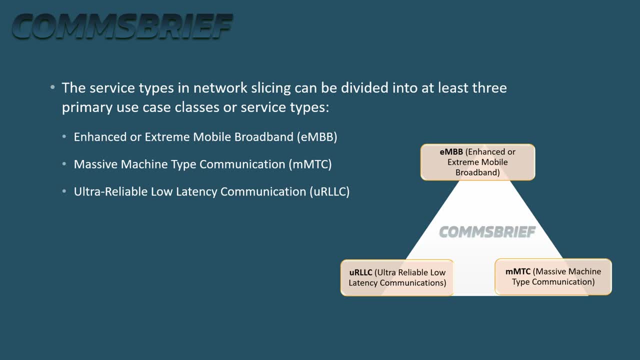 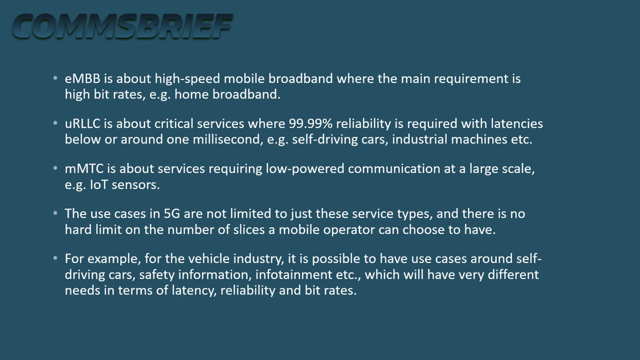 three primary use case, classes or service types: Enhanced or Extreme Mobile Broadband, Massive Machine Type Communication and Ultra-reliable Low Latency Communication. EMBB is about high-speed mobile broadband where the service type can be divided into. the main requirement is high bit rates, for example home broadband. 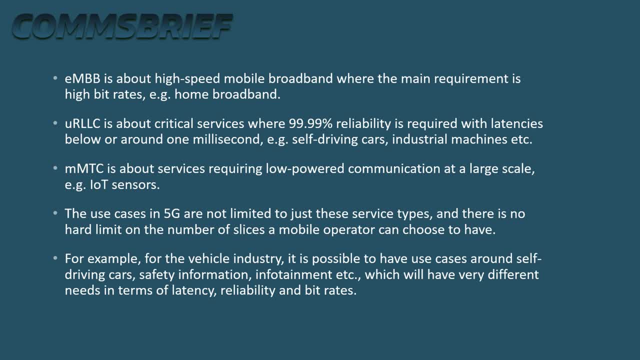 URLLC is about critical services where 99.99% reliability is required with latencies below or around 1 millisecond, for example, self-driving cars and industrial machines, etc. MMTC is about services requiring low-powered communication at a large scale, for example. 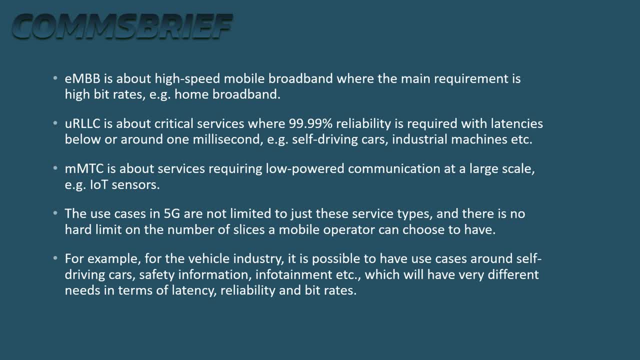 IoT sensors. The use cases in 5G are not limited to just these service types and there is no hard limit on the number of slices a mobile operator can choose to have. For example, for the vehicle industry, it is possible to have use cases around self-driving cars safety information. 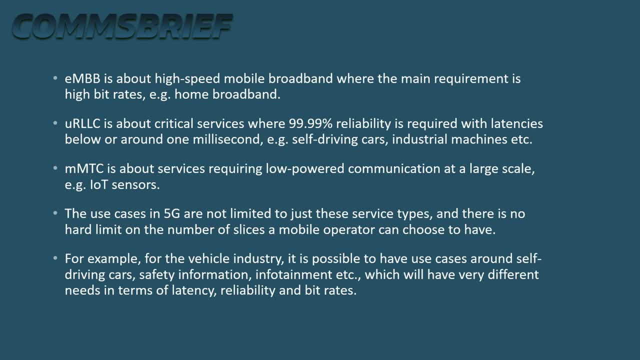 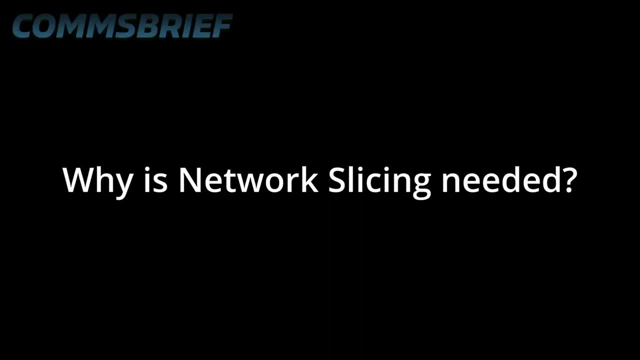 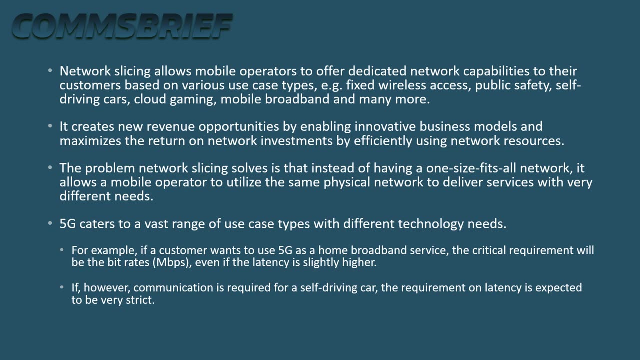 infotainment, etc. which will have very different needs in terms of latency, reliability and bit rates. Network slicing allows mobile operators to offer dedicated network capabilities to their customers based on various use case types, for example, fixed wireless access, public safety. 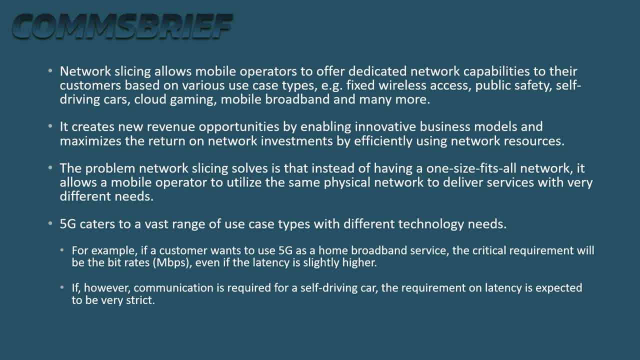 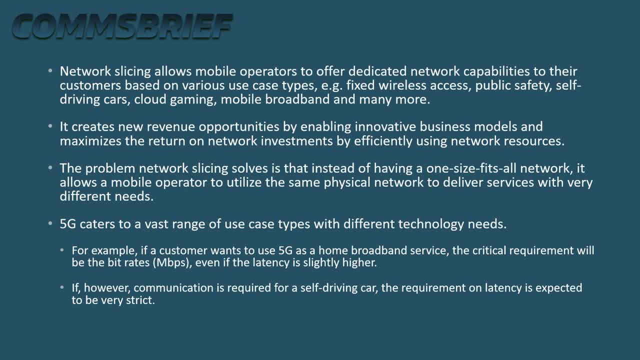 it is not possible to use the network as a whole, but as a whole. The problem network slicing solves is that, in still-time, in still-time, a one-size-fits-all network allows a mobile operator to utilize the same physical network in order to deliver services with very